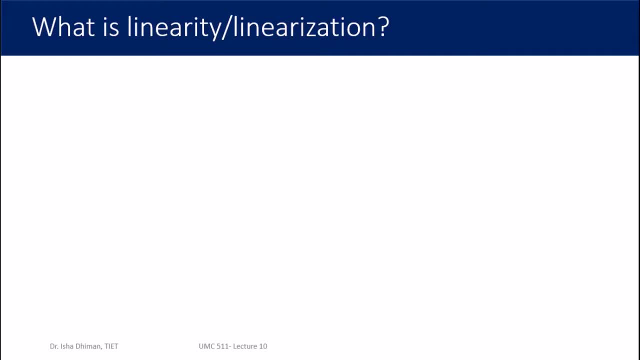 and subtractions and the scalar multiple of the variables are allowed. So we already have much idea about the linearity and linearization. So there is, as such, no formal way, but theoretically speaking, linearity means the presence of linear expressions and linear terms in our model. However, it can depend on the context of problem as well. For example, if you look at this: 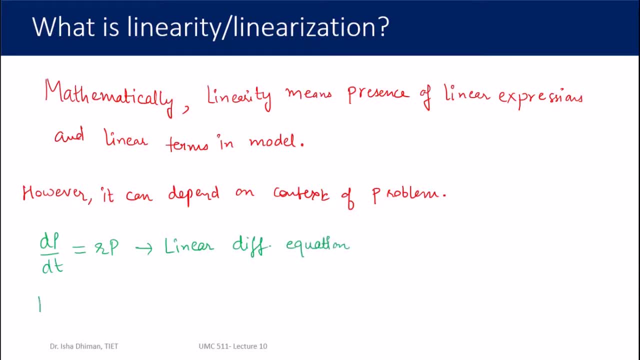 model dp by dt is rp. this is a linear differential equation of first order and its solution is an exponential growth. Therefore, the model is also called exponential growth model or exponential model. We have already discussed this model in detail when we were studying the population growth. 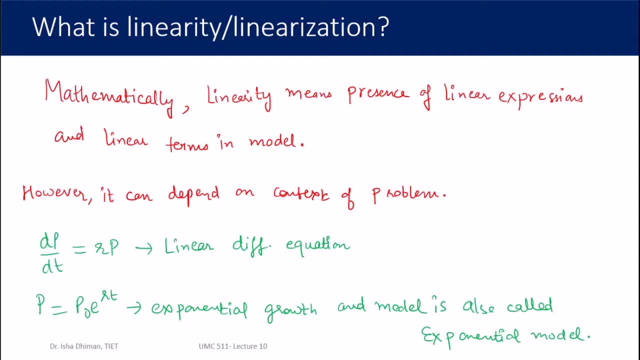 models. So, as a differential equation, this is a linear differential equation because you can see, it's just a scalar multiple of p. there is no p square or p cube or not multiplication with the dependent and independent variable. So nothing like that is there. So that's fine. So let's. 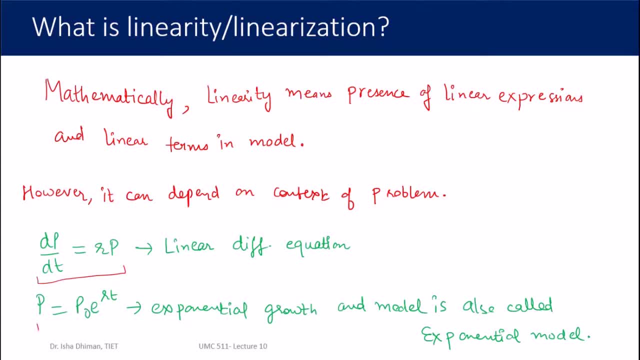 apply as a differential equation. this is linear. However, if you look at its solution, then that's a exponential profile. That's why the model is called exponential growth model or exponential decay model. depending upon r is positive or negative, So the model is deriving its name from. 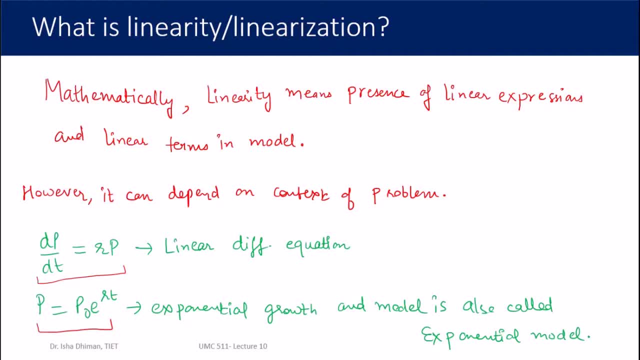 the solution, but as a differential equation. the definition of linear differential equation. if you apply over it you will get to know it's a linear differential equation. So in the language of or modeling as such, there is no fixed way of defining that this is a linear model and this is a nonlinear. 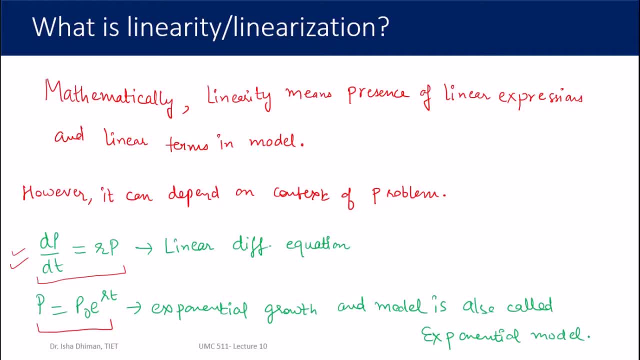 model. It really depends on what context linearity we are talking about. Are we talking about the differential equation or we are talking about the solution? So that can vary. So that's why I just want to explain you here that you may get confused with some models, that there should not be ambiguity. 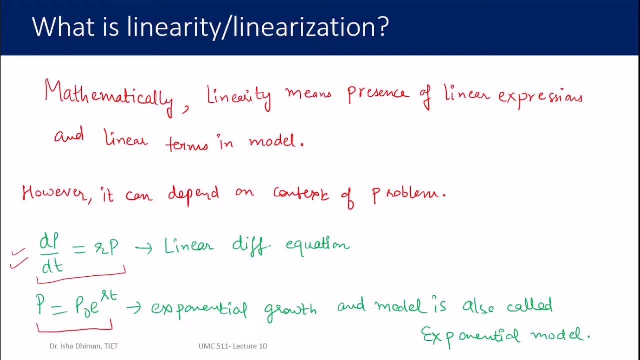 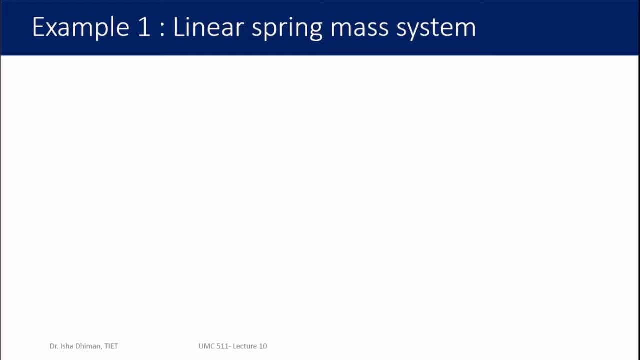 or there should not be confusion in that, And I just think I have already explained that, So I will explain this point in the previous lectures as well. So that's a general idea about linearity. Now we'll do certain examples of linear models. Example 1: I have picked a very simple example to 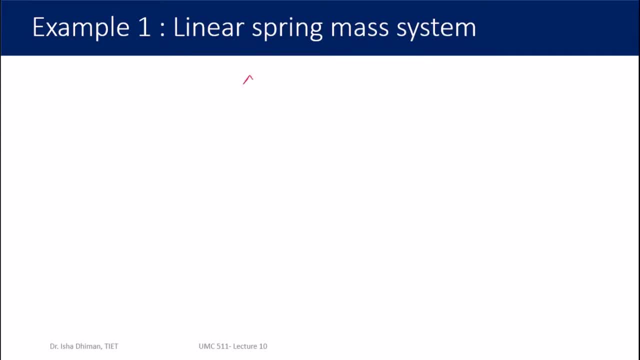 begin. It's a linear spring mass system. So you have a spring and a mass m attached to it and in the x direction you are giving the displacement. So you know how the spring mass system works. So this is a linear spring mass system. So you have a spring and a mass m attached to it and in 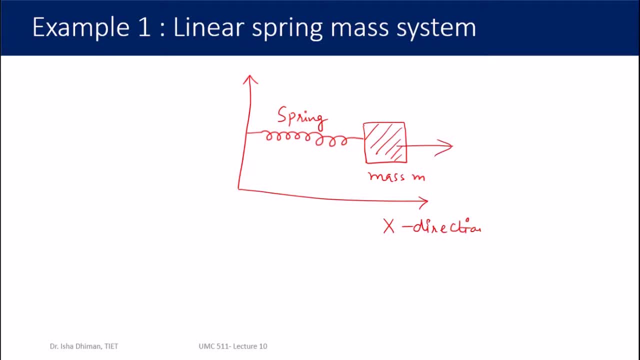 this mass m if you give it displacement in this direction. So obviously you displace it up to certain point x from its center position, say whatever is the equilibrium position, You displace it and then it will come back to its original position and it will keep on oscillating. 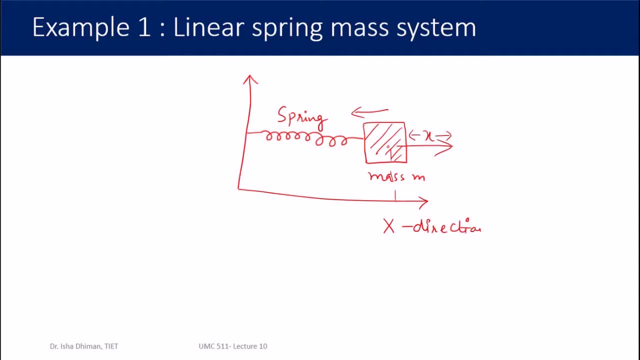 because of the spring, because of the inertial force, because of the force applied there. So we want to write a mathematical model for this spring mass system. So if you apply Newton's second law, so we know that the force is mass into acceleration. So m 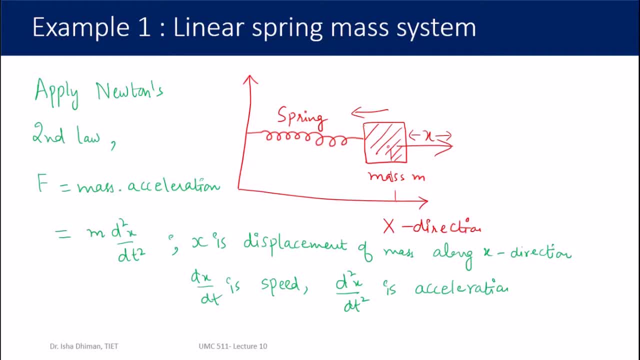 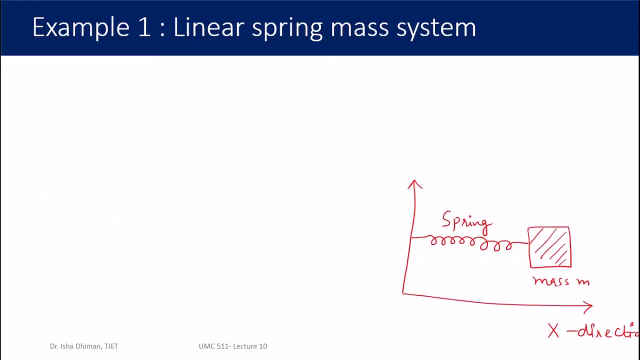 into d2x by dt square, because x is displacement, So dx by dt is speed, So d2x by dt2 is the acceleration. So we know that the formula for force applicable on the mass m is given by this and we know that that this is proportional to x, directly proportional to the displacement. 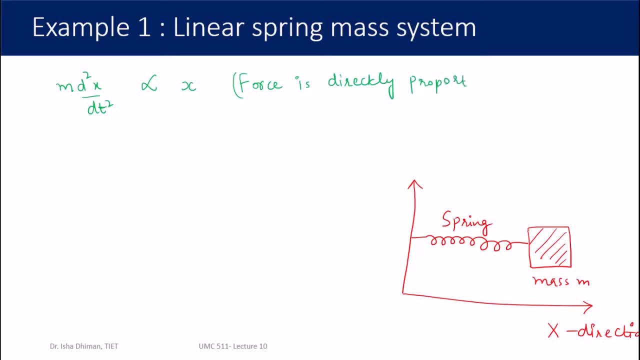 because larger the value of this, this displacement, is, stronger the magnitude of this force is going to be. So because of this direct proportionality, we are getting linearity into the system. So that's another way of looking at linear. whenever you are measurable, quantity or whatever physical quantity in your observation is proportional to something the your. 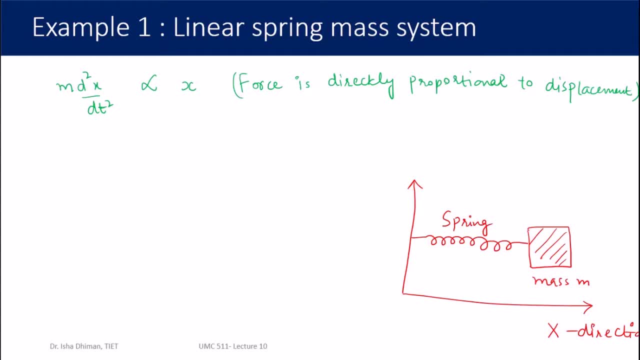 variable Like it's proportional to x. So obviously when you remove the sign of proportionality and replace it with equation, it will be giving your constant of proportionality. so K is here constant of proportionality, which is called the stiffness coefficient or the stiffness constant, and it really depends on the 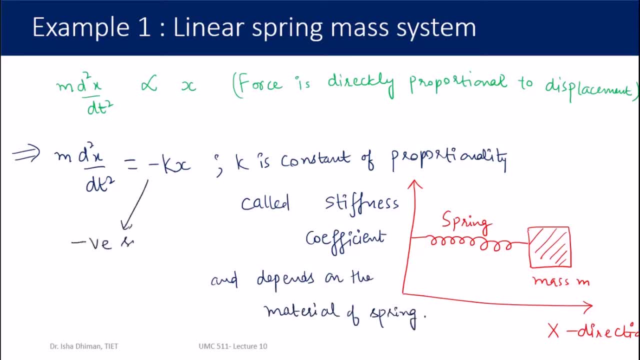 material of the spring used and negative sign indicates that this force gets applied in the opposite direction of displacement. so it's very obvious, the ways I've just explained to you, because you are giving the displacement in this direction, the force is being applied in this direction, that that force is. 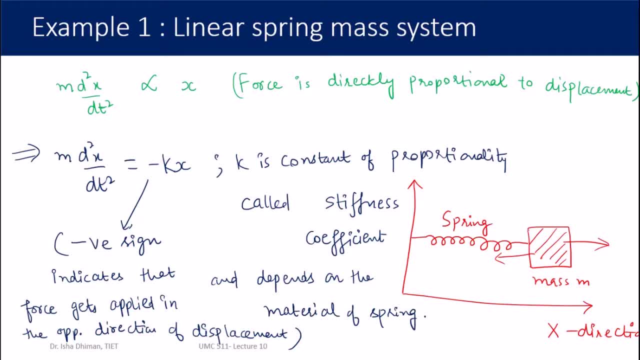 responsible for pulling it back into its direction and giving its oscillation. so that's why negative sign is there. so because of this factor, K into X, so it's just a scalar multiple of X. there is no term like X square or something like that. that's why this factor is responsible for the linearity of this. 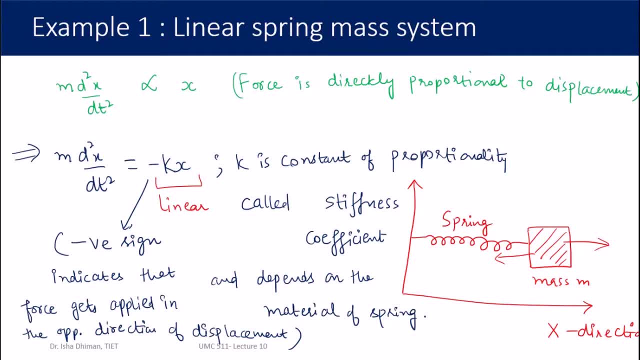 factor model. so it's. it's not like it's never like that. we assume linearity. in some cases we have to assume the linearity, but in most of the cases the linear models work so well that they are actually replicating the dynamics of the 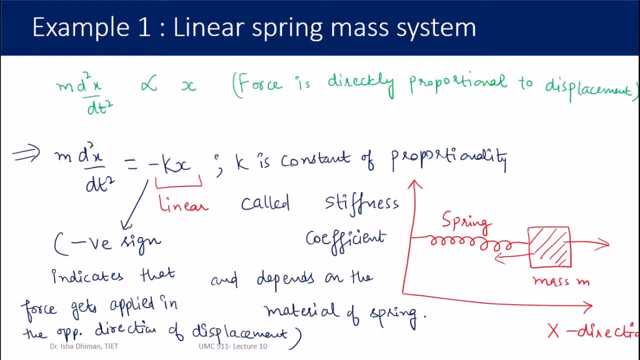 real system they are usually. it's said in the subject of mathematical modeling that a nonlinear model is always better than the linear one. it might be true to some extent, but for many of the example the linear versions of the model also work very well. so because of this direct 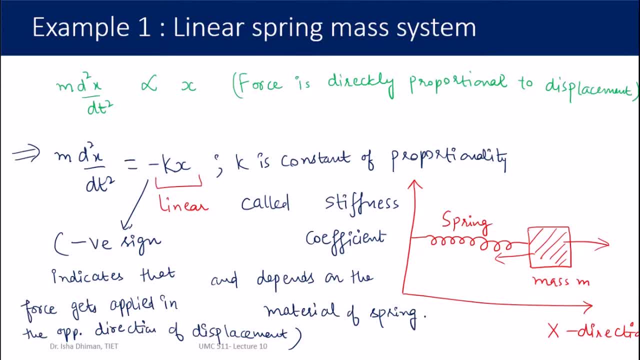 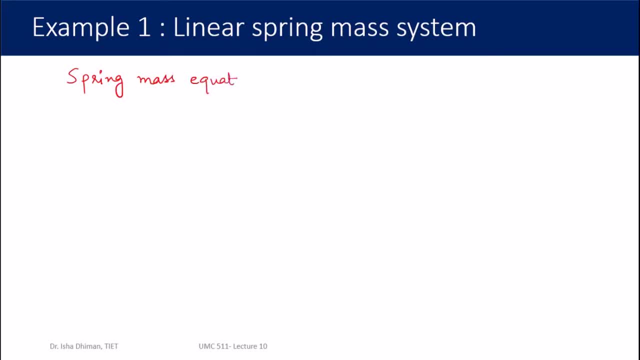 proportionality. the linearity is arising over here. so we get a differential equation which is called spring mass equation: M, d2, X by dt2 is minus kx. it's a linear, second-order differential equation. so now, if you talk about solving it, so we can solve it by putting dx by dt is. 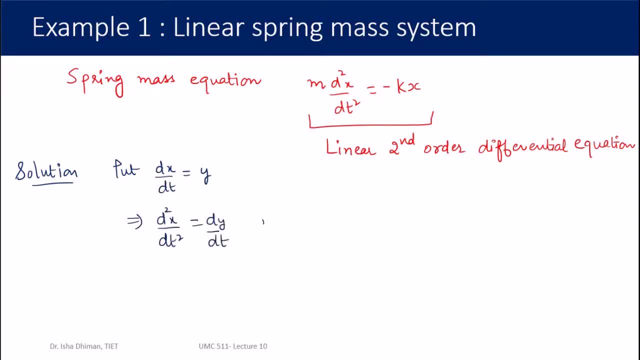 another variable, Y, which will give you d2. X by d2 is dy by dt. if you substitute this, you will get M: dy by dt is minus kx and dx by dt is y. so this is a coupled linear system of first-order differential equations. first-order: 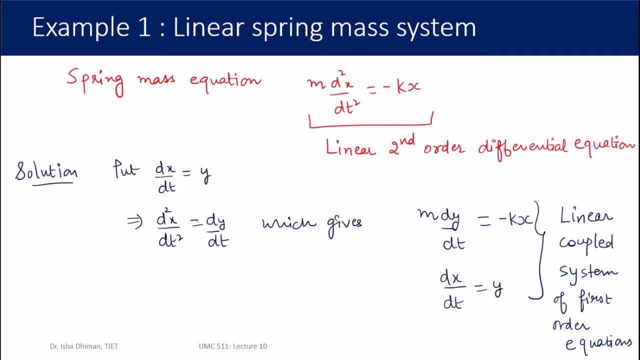 ordinary differential equations, because the original model is a second-order differential equation. so one of the way of solving is you couple the system. you convert the one second-order differential equation into a system of two first-order equations. so that's one way, and now this is a coupled system. coupled means you can see Y is a. 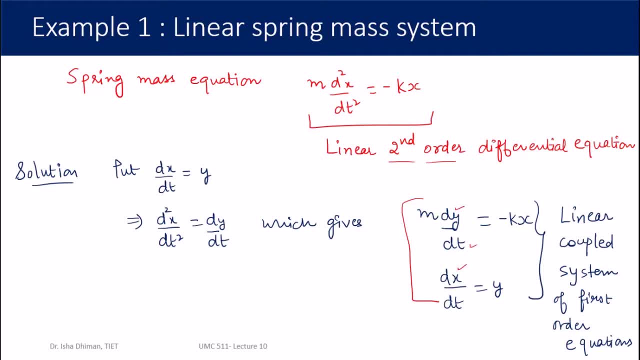 dependent variable. X is the dependent variable and T is the independent variable. so both X and Y are functions of T. so in this equation X is a pair and in this equation Y is your pair. so you cannot just solve this equation separately and saw this separately and then combine. you have to. 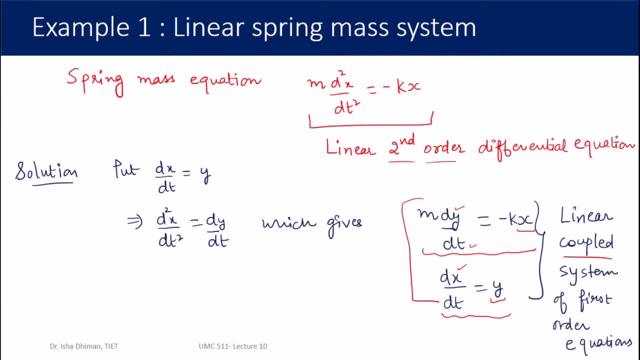 solve this simultaneously. that's where the coupled system. so that's one way of getting the solution. you solve this system of equations or other ways. it's simply coming from the way you have learned in your earlier courses that how to solve linear second-order differential equation. so you can do. 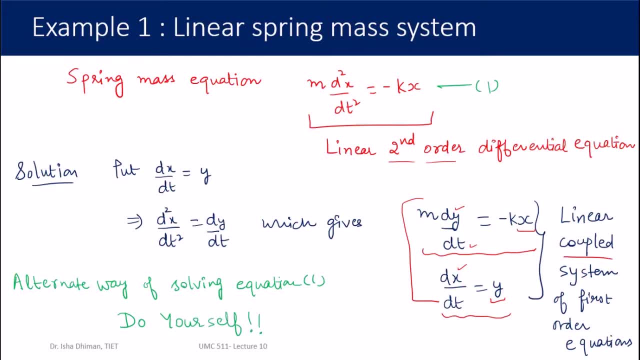 that yourself, because right now theтеx- and they are in different Mmmm- that how to solve linear second-order differential equation. so you can do that yourself, because right now now the aim of this lecture is not to tell you how to solve a differential equation. that part. 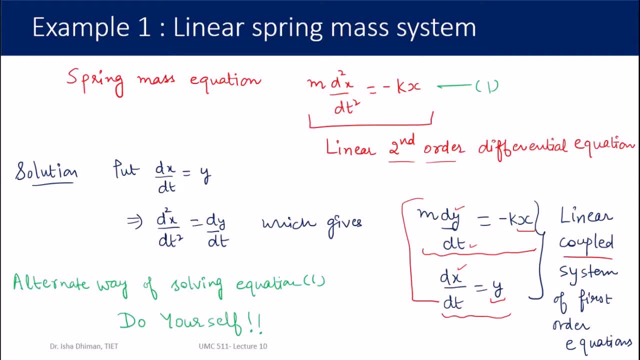 you have already studied in your early classes, so i won't be doing that again over here. you can do that again. learn yourself right now. in this lecture we are just focusing on the understanding of linearity and the examples of linear models. so very easily you can solve this model and then 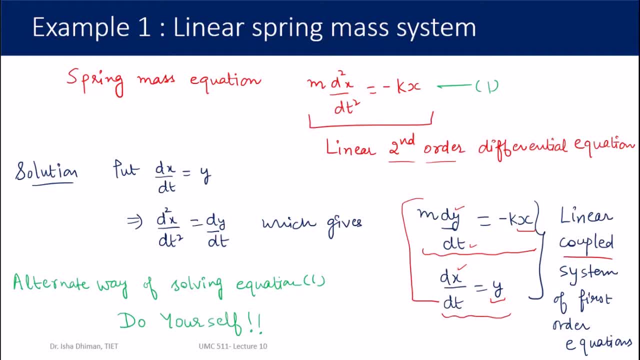 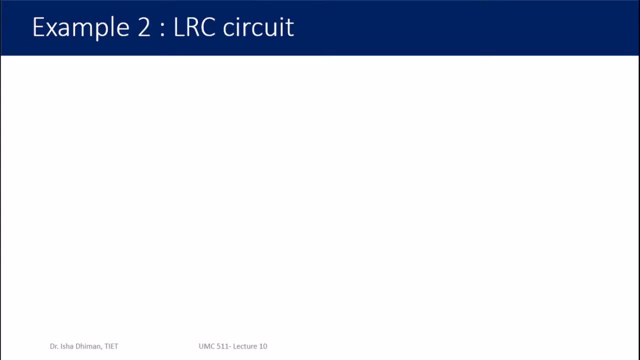 you can try to interpret the solution that, with the presence of linearity, what is happening in the solution? let's begin to next example. again, it's a very simple example. all of you are very much familiar with it. it's a lrc circuit, so if you draw a diagram for it, so we have a resistor. 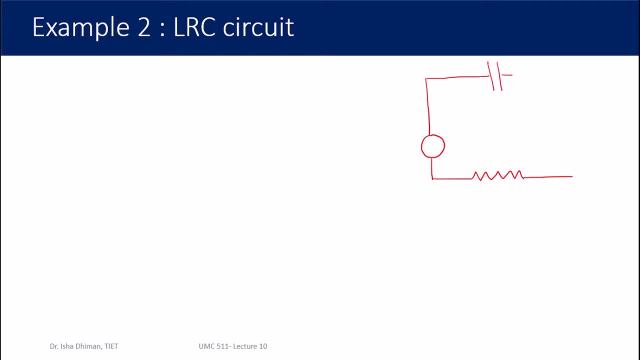 into the system. we have a capacitor and an inductor. so inductor is with the inductance l, capacitor is with capacitance c and resistor is with the resistance c and and, and there's obviously a voltage supply, the supply of electricity into the circuit. so we want to apply Kirchhoff's law, because in previous example we 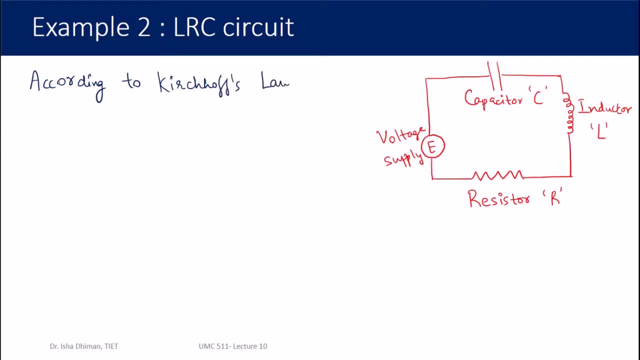 apply Newton's law. so here we will apply the law of Kirchhoff, which tells you that the sum of voltage drops across all the circuit elements is going to be constant. because that should be actually constant means that should be matching with your electrical supply which you are getting into the system because of. 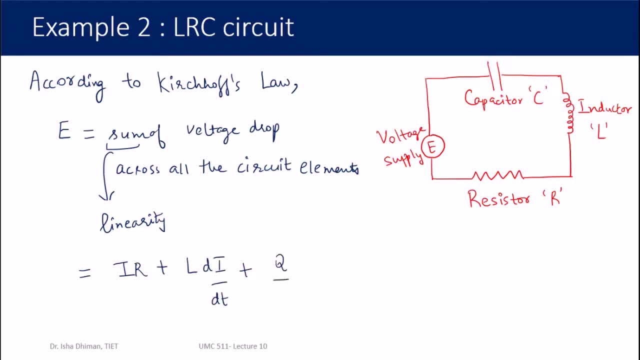 conservation. so it is sum of three terms: IR plus L di by dt, plus Q by C, where Q is charge of the capacitor. so IR is the voltage drop across the resistor, L di by dt is a voltage drop across the inductor and Q by C is a voltage drop across the. 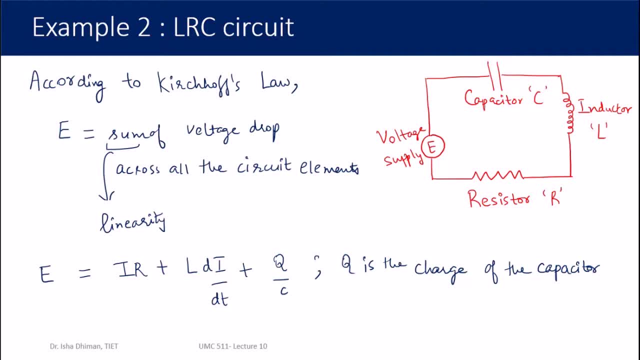 capacitor. again, I'm not going to explain how these expressions are coming. you all have started in the basic electronics in your 12th standard class that it's very easy to look at. these are just coming from the basic formulas of the circuits. so if you look at that expression again, so applying Kirchhoff's- 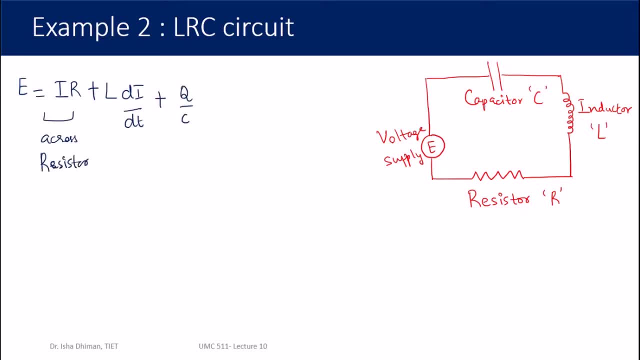 law we get here. so that's across the resistor, that's across the inductor and that's across the capacitor. so now we know that this- I, the current- is dQ by dt, because that's just the basic definition of current. it's the rate of change of charge. so you replace that into your. 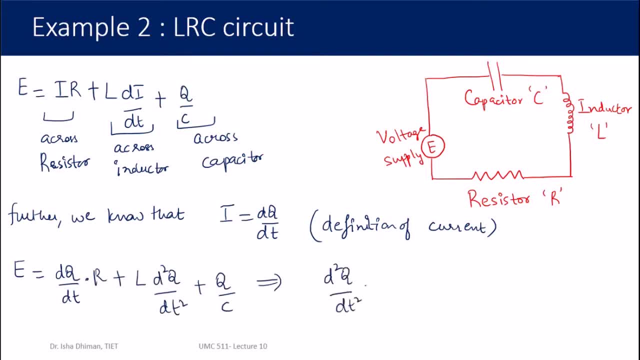 equation you will get this dQ by dt2 plus R by L, dQ by dt plus Q by C. L is E by L, which is also a second order linear differential equation which also I'm telling you to solve yourself. So it's very easy to understand. 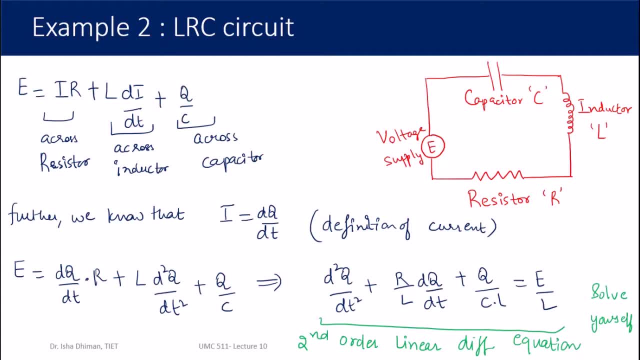 easy to solve. so here also, my purpose was to tell you the linearity. so what bring linearity into the system here? which assumption did bring linearity into the system? the assumptions and these applications of ohms law. basically, ohms law is also, if you remember, what is ohms law? so this: 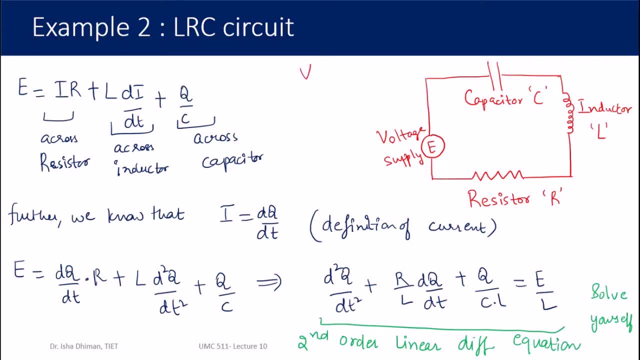 voltage. you know, the ohms law just tells you v is equal to i into r, because it assumes linearity, that v is directly proportional to r. or you can say it in other words: but because of this direct proportionality with r, there is no r square or there is no other power of r. because of this. 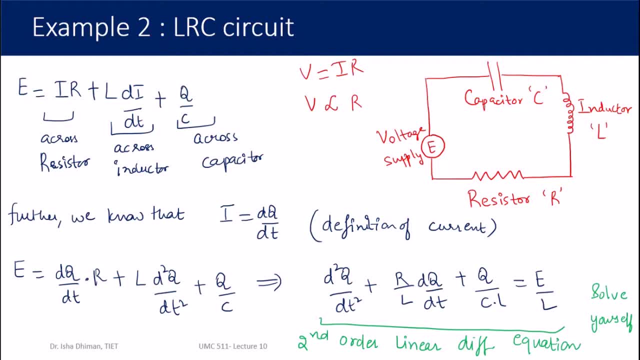 direct proportional. with the linear power of a factor or of quantity, we get the linearity into the system. so same is for capacitor and inductor. so because of their individual linear expressions the sum of linear is also linear. there is no product term. so that's why. 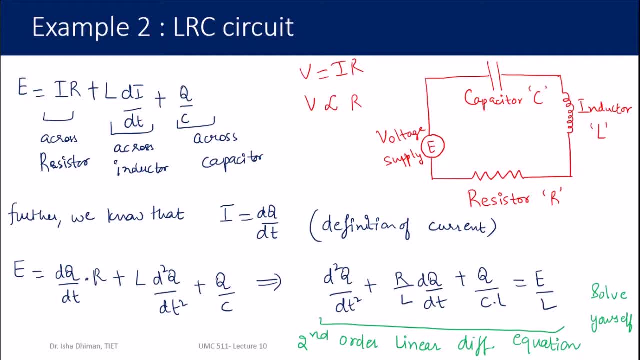 over Overall, the expression becomes a linear expression and this is just the definition of current when you use it. So you see that, because this R, L and C are just constants, They are not. you cannot assume or you cannot interpret that they are coming as a product term. They are just constants. 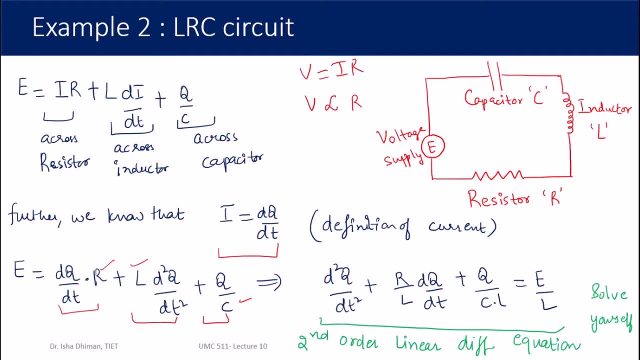 They will have fixed values. We just need to focus on the dependent variable. So the dependent variable is finally Q. Earlier this was I, but Q was also there, So we also shifted I in terms of Q. So finally we have just an ordinary differential equation, because we have just one independent. 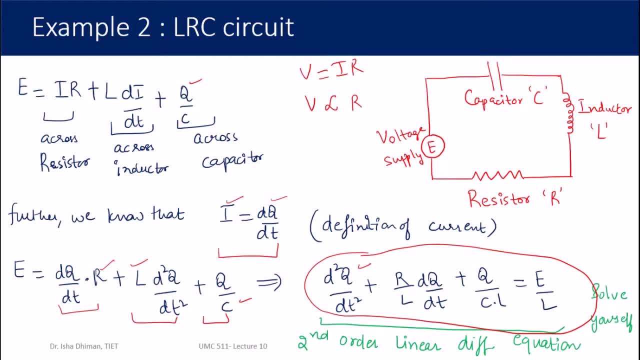 one dependent variable and one independent variable. So that's your. the consequence of linearity is there, which is giving you this equation, and this equation very well explains and captures all the dynamics, or all the you can say how to do it. So this is the definition of a linear expression. 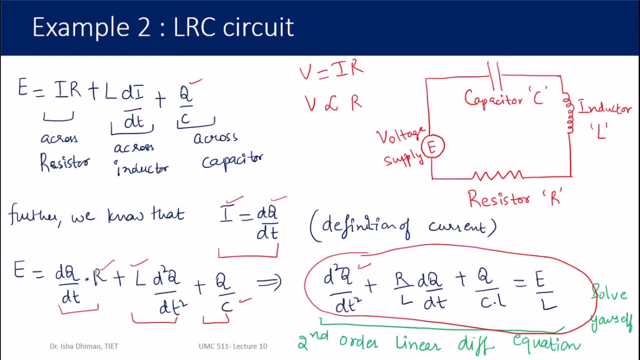 So this is the definition of a linear expression. So this is the definition of a linear expression: How the current is flowing through the system, how the voltage is passing across all the elements. So it's very well captured. So again, an emphasis is being given on that, even the linearity is. 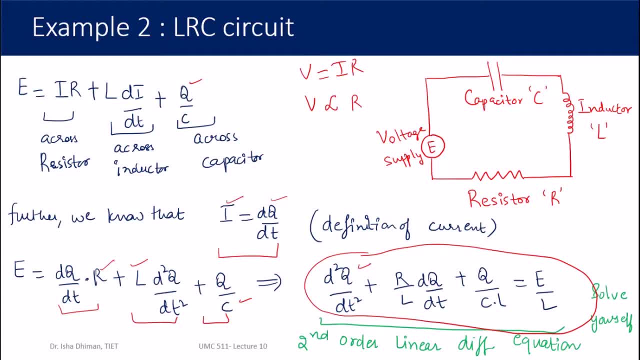 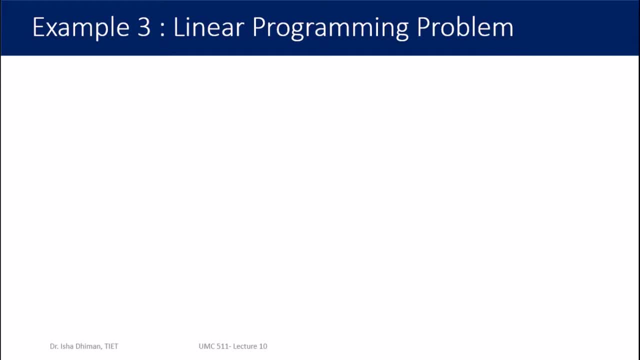 capturing the system dynamics very beautifully. The third example which I'm going to take is all of you are already familiar with. It's an example of a linear programming problem, So you can just recall it quickly. We know how LPP looks like. 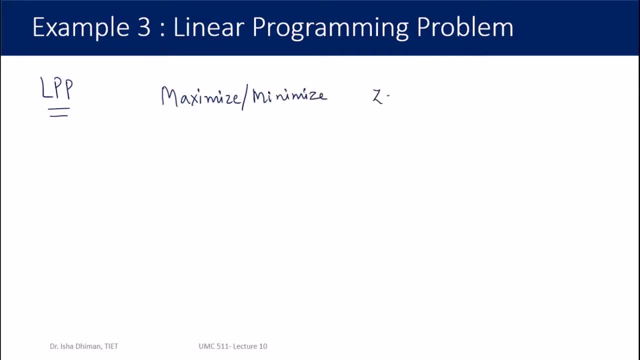 Maximize or minimize some Z equals to C. transpose X subjected to AX equals to BX, non-negative. So your C is the cost vector, X is your unknown decision variable vector and A is your coefficient matrix, having M constraints into the system and B your resource vector, the right hand side vector. 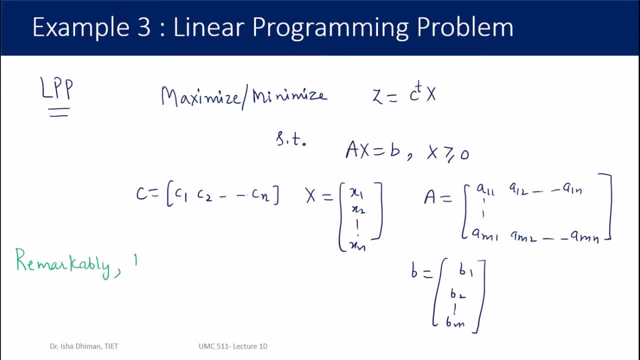 So remarkably, we know that this LPP Are able to work quite well For industrial and business problems Because you see, a variety of problems we have discussed in that course of optimization techniques where most of the cases, most of the industrial examples, be it a transportation problem, be it a supply chain problem, be it an assignment problem, job assignment or whatever the different kinds of problems we had, all of them were able to work quite well. 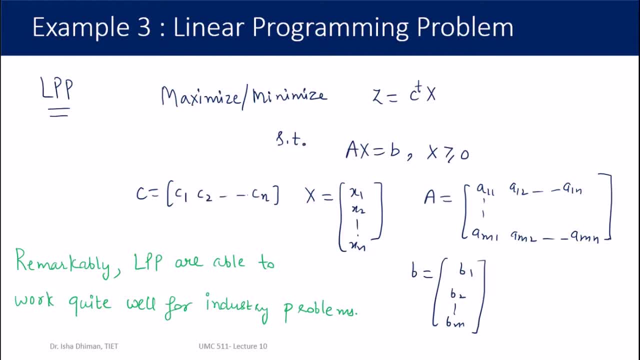 So that's another good example of understanding that how the linear models are going to be very much successful in giving us good answers. So there also, although the system was large, but whatever was present in the system was all linearity. So that's another good example of understanding that how the linear models are going to be very much successful in giving us good answers. 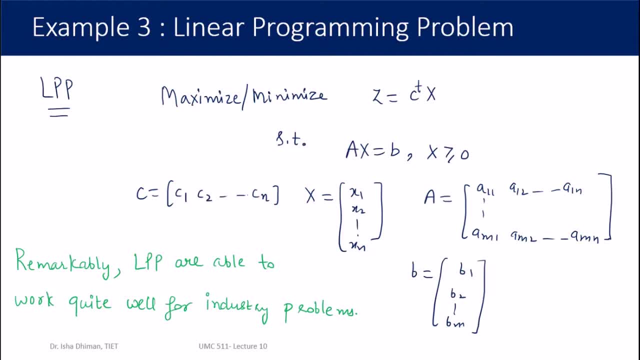 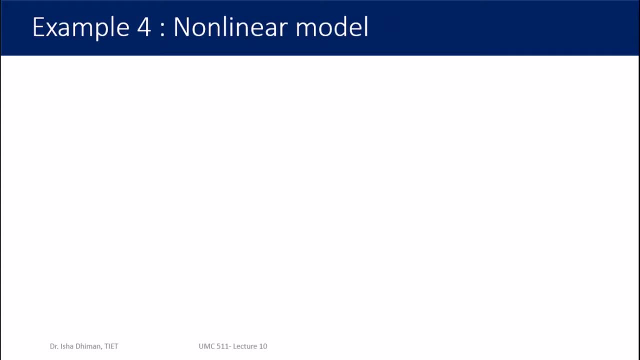 So that was the third example. I'm not going into details of this. That was just to tell you that this is one example of linear models. Next example I'm going to take is a nonlinear model, And so for that we have to take the example of a pendulum. 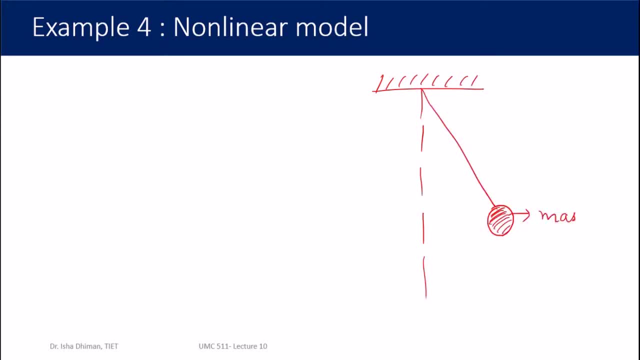 Having mass m, length l and making an angle theta, obviously you give the displacement through an angle theta. This is the forces acting, the gravitational force mg, If you split it into two components: one along the perpendicular direction and one along the other direction. 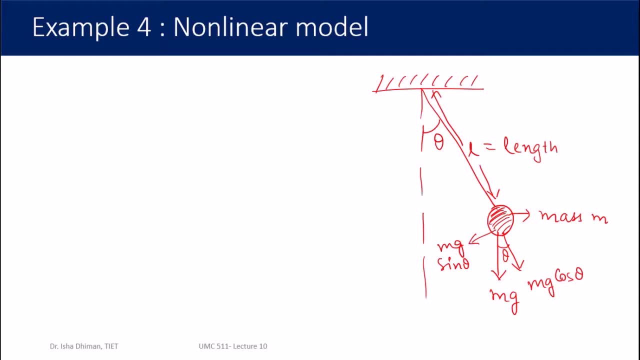 We know that This is how you break the forces. One component will be mg sin theta. Another component will be mg cos theta. So we know why this is cos theta: because if you use this law over here, So this is going to be mg cos theta, because this theta is angle, because this theta is angle. 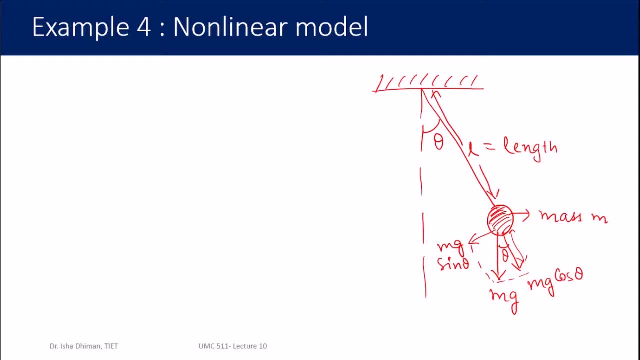 So once you get this splitting up of force components, then we know that if this is the displacement- Suppose this is the original position- And s is the angular displacement- Then we know that s is l into theta And force is mass into acceleration: t2, s by dt2.. 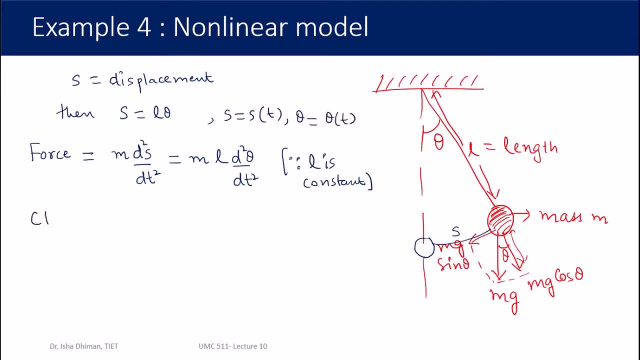 Which is ml d2 theta by dt2.. So clearly, this is minus mg sin theta, because we are balancing the force perpendicular to the pendulum, And this negative sign because it's a restoring force. So what do you mean by restoring force? It's similar to the spring mass system which we have just studied. 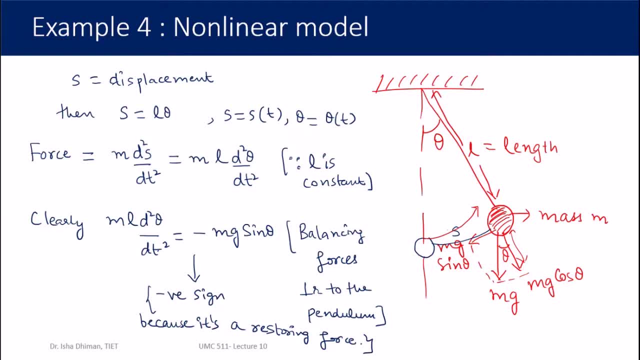 Because you give displacement in this direction and the force acting in this direction. You can see this mg sin theta is acting in the opposite direction of the displacement, So it's bringing it back to its equilibrium position, It's trying to bring it back to its equilibrium position. 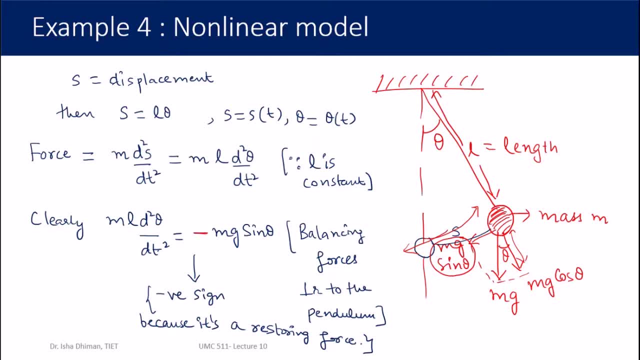 So that's why it acts in the negative direction. So the negative sign is because of that And s is l theta we have used here, because l is constant. So s is a function of time, because the displacement is obviously changing with respect to time. 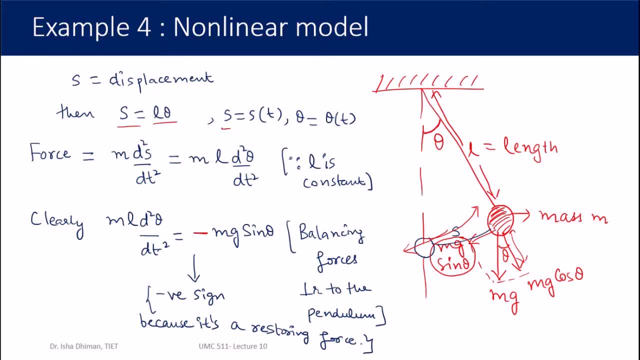 Theta is obviously changing with respect to time, So they are both our function of time. That's why we can write it like: d2. s by dt2 can be written like this, And when you replace it over here, you get this as your equation: 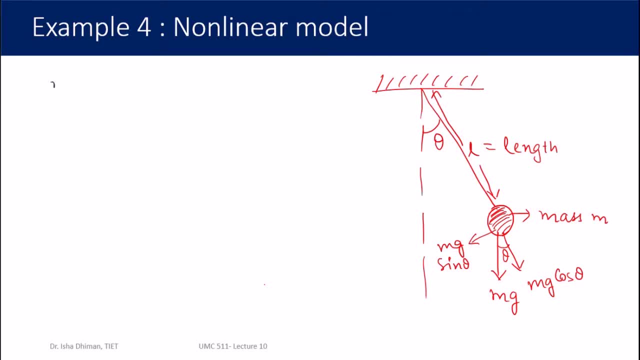 So finally we have this equation in front of us: ML d2 theta by dt2 is minus mg sin theta. You take the terms to one side. d2 theta by dt2 is minus g by l sin theta, Or you can write it this way as well: 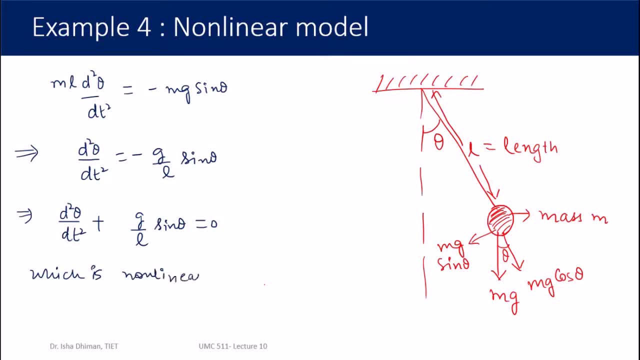 So now this is a non-linear differential equation Because of the presence of transcendental function, sin theta. I told you in the beginning the presence of these kind of functions, trigonometric, logarithmic, exponential functions, These make the things non-linear. 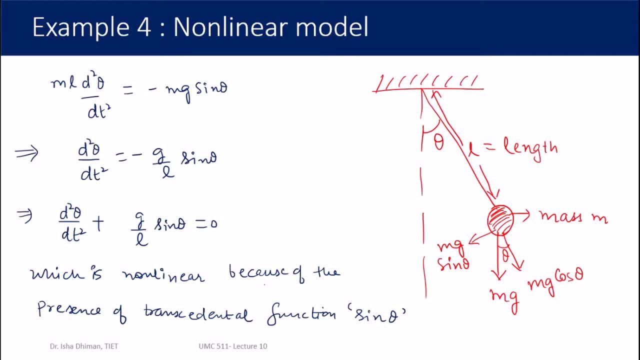 Because these are not considered in the category of linear functions, Because their behavior are not of the linear functions. So this is a non-linear mathematical model explaining the dynamics of this simple pendulum. So now, what further we are going to do? I will rewrite the equation once again. 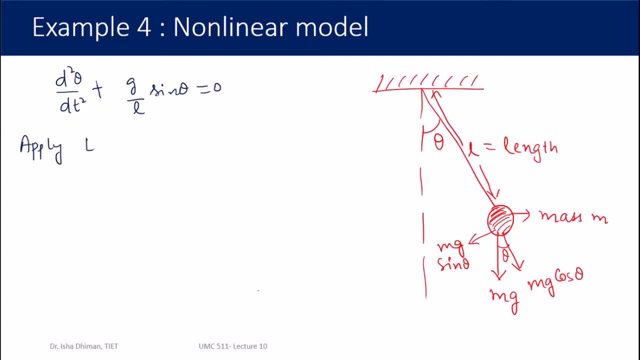 And now I will apply the technique of linearization to this equation to get a linear version of the same model. So how to do that? So we know that sin theta is approximately equal to theta when theta is small, measured in radians, of course. So you use this. 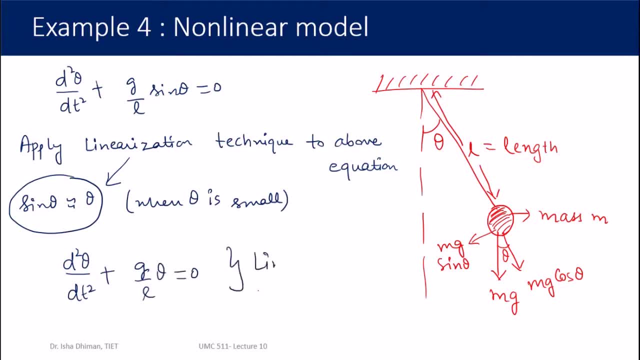 You get g by l, theta equals to 0. So this is nothing but linearized pendulum And it works quite well. again I will say when theta is small. So the original equation was having a factor of sin theta, But our approximate equation is having theta in place of sin theta. 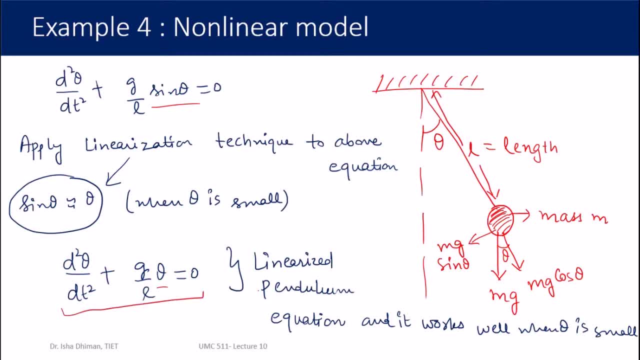 So that's obviously an approximation of our original model. Or you can say it's a linearized version of the original non-linear problem. So the solution of this will be an approximation. This will be an approximate solution of the original problem. But we know that this approximation is going to work very well when theta is going to be small. 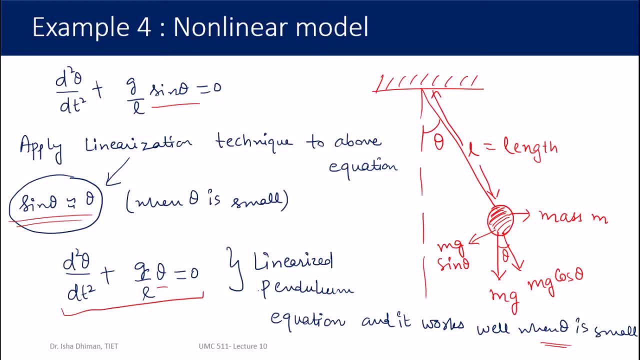 So that's the benefit of linearization. Why we do linearization? Because we know that our mathematical techniques of solving or dealing with the linear equations- Be it linear system of equations, algebraic equations or be it linear system of differential equations- We know that linearity is always easy to handle. 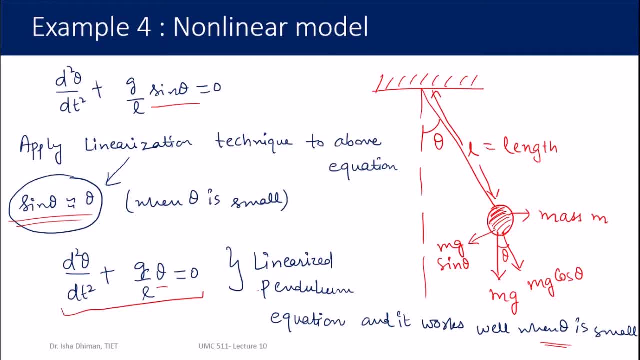 We do have well defined mathematical techniques for dealing with linearity. But to deal with non-linearity things become difficult. We have to apply the numerical techniques there, Because there are very less number of analytical techniques for the non-linear problems. So therefore everybody just wants to get rid of the non-linearity somehow. 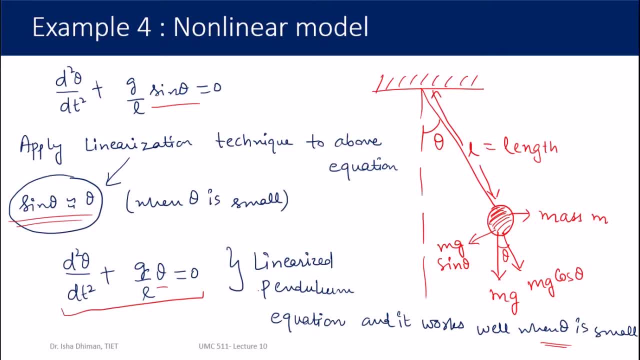 And that's the rule in mathematical modeling Whenever you are formulating a model And that turns out to be a non-linear model. So the very first attempt we make to solve that is okay. Let's first solve the linear version of it. 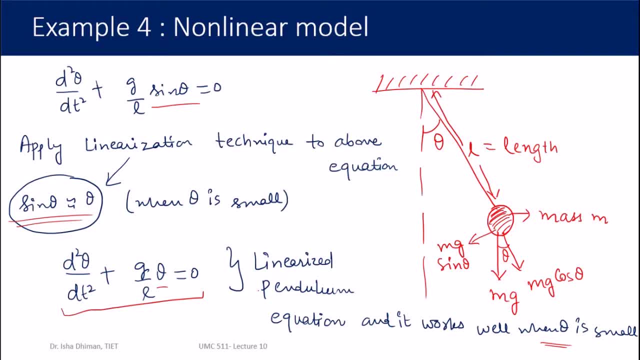 And then try to see how much good or poor approximation that is giving. So that's why it's very important to learn the technique of linearization in mathematical modeling. So this was very simple example and probably we have done this in our earlier classes also. 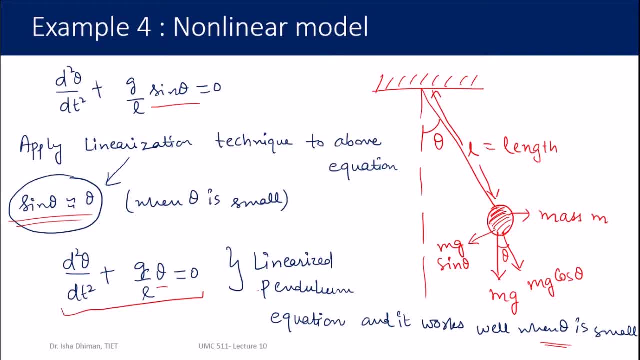 Maybe we were not aware with the term that we are doing this as a linearization, But this is kind of an approximation which we are using. So what happens next? We can solve this again yourself, So I am not going to the detailed solution of it. 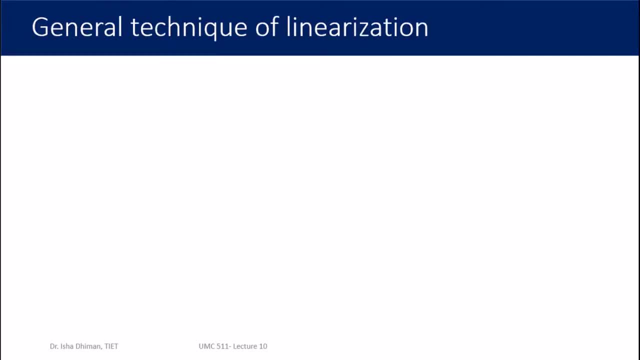 So with this example, you have learnt a way of linearizing That you replace the sin theta with its theta. So there should be a general technique of linearization. So let's try to learn that. So why we did so in the previous example? 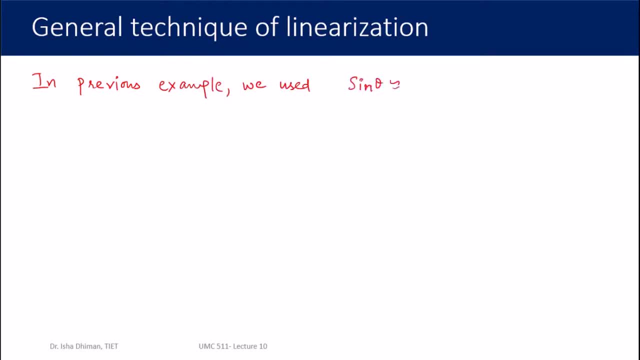 So we used sin. theta is approximately equal to theta when theta is small. So basically I used the, if you recall, Taylor series expansion of sin x. I can write the Taylor series expansion of sin x because that's a smooth function. So it's x minus x cube by 3 factorial, plus x raised to the power, 5 by 5 factorial and so on. 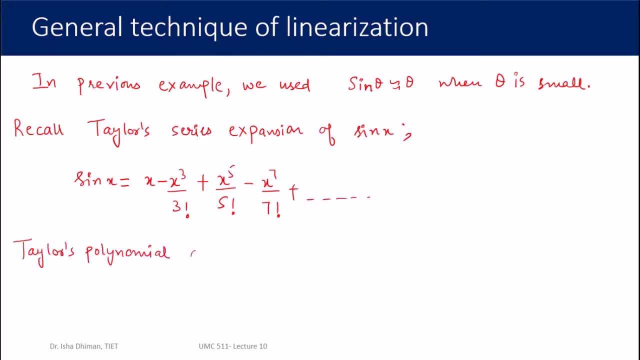 If I ask: what is the Taylor polynomial of 1.. So that's nothing, but it's just one term, x, And of degree 3. it's these two terms And so on. So it depends upon what order or what degree the Taylor polynomial they are asking for. 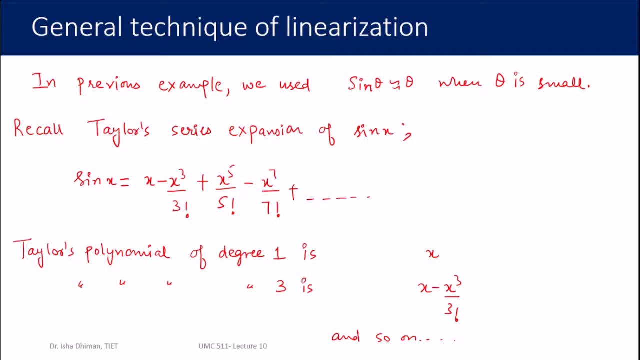 So you can write this. So why I am focusing on these things? because these Taylor polynomials are the approximation. So a linear approximation will be just this much, While a second or sorry, a third degree approximation will be up to this term. So, since we are just doing with the 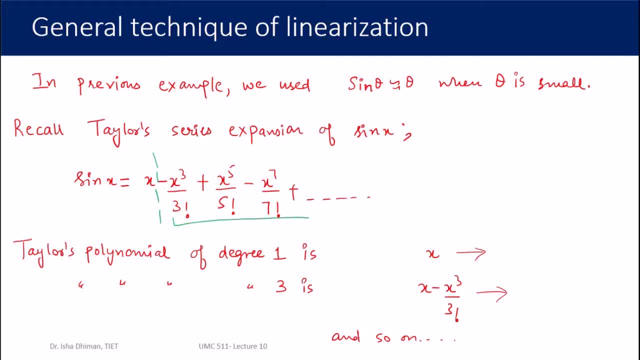 Linear one, So we have to have it like here. So this is an error term If you truncate at x. So clearly, if x is small, then error is also small. Therefore, sin theta is approximately equal to theta for very small values of theta. 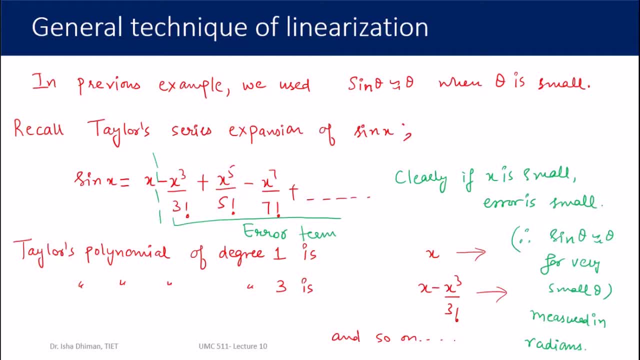 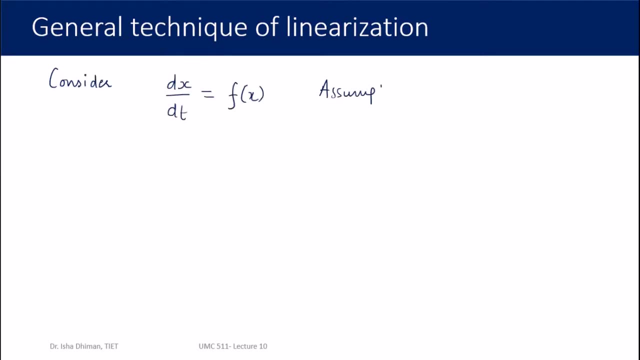 So that's the idea. You have applied indirectly Taylor series approximation in the previous example While using that approximation. So now I will give you a general way of doing that. So you consider a general equation: dx by dt is fx. Assumption f is a smooth function. 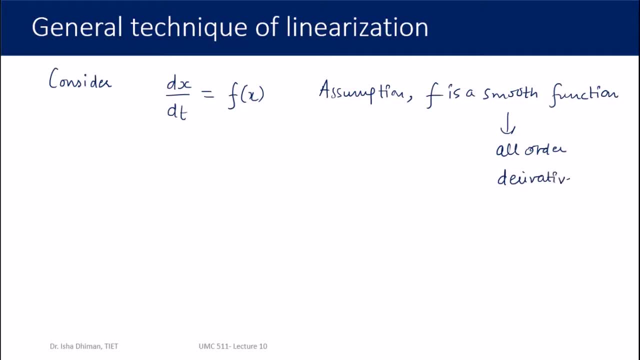 Because smooth function means it's all order derivatives are existing So that I can expand the function as Taylor series. You can have an example of smooth function is a exponential function, e raised to power x. So you write the functions fx, Taylor series: Expansion about certain point: x equals to a. 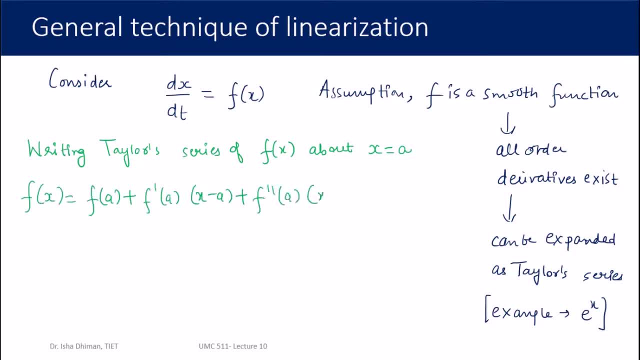 So we know this is the Taylor series, fx is fa plus f, dash x minus a plus this term and so on. So this one is just the linear approximation, Because up to first degree we have to consider and rest of the terms you have to ignore. 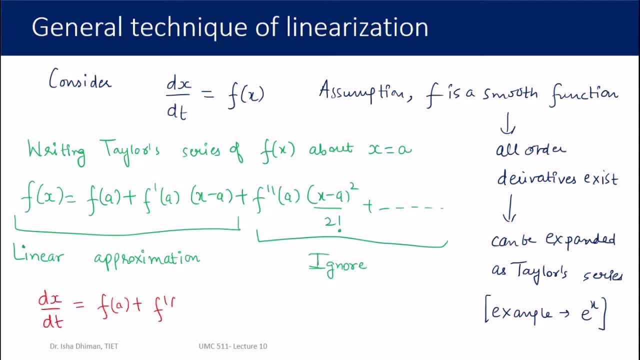 They are higher order terms. So dx by dt is fa plus f, dash x minus a. So I have replaced fx with its linear approximation. Now we just need to do a little bit more calculation. So this is your original equation: dx by dt is fx. 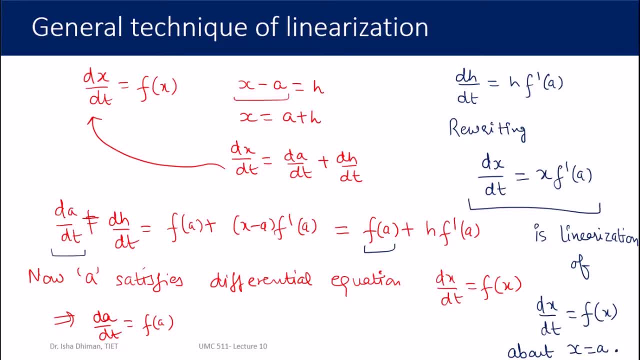 So x minus. a term is coming in your approximation, I am putting it equal to h. So x equals to a plus h. So you differentiate this with respect to time. You will get dx by dt- is da by dt plus dh by dt. 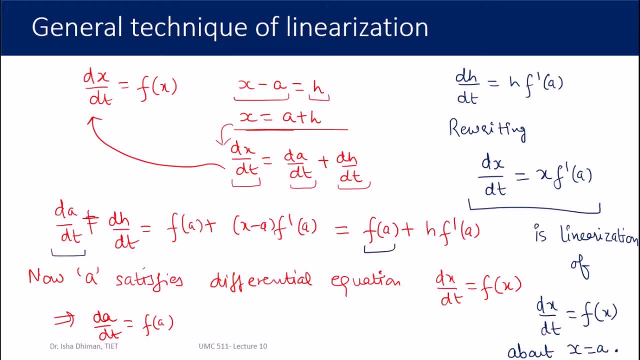 And if you put this value here You will get da by dt plus dh by dt. So dx by dt is fa plus this, While we know that a satisfies the differential equation, Because a is one of the- you can say- solutions of the differential equation. 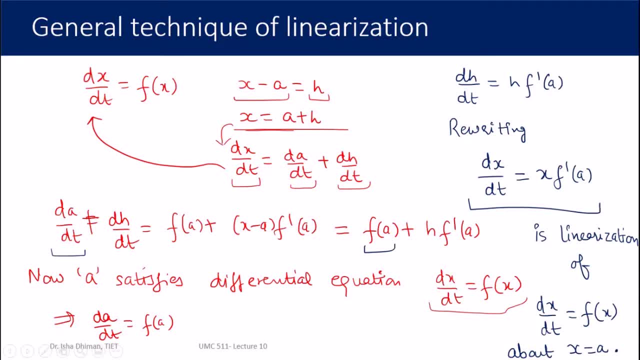 That's why we are able to expand it around that So da by dt is f of a, So da by dt is f of a. So this term gets cancelled And we get here: dh by dt is h times f dash a. It's very easy to calculate. 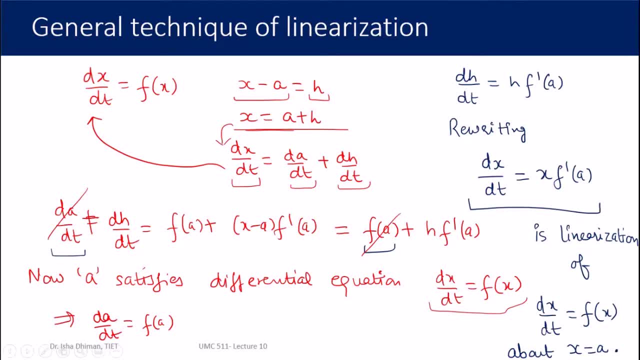 So this is our. if you rewrite h as x, You will get dx by. dt is x times f dash a. So this is the linearization of this about x equals to a. So that's the general way. You don't need to remember this as a formula. 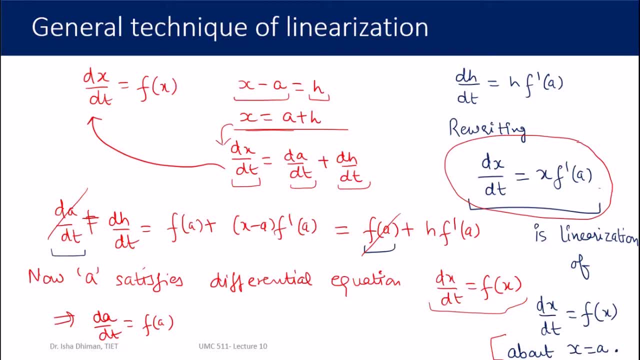 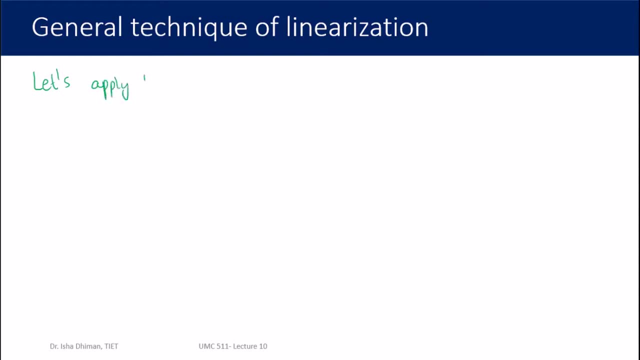 But still we can. if you can remember, then you can remember. Otherwise, simply always understand that we have to apply the Taylor series And keep the terms up to first degree for linearization. So this technique, if you apply Over the same example, sin theta. 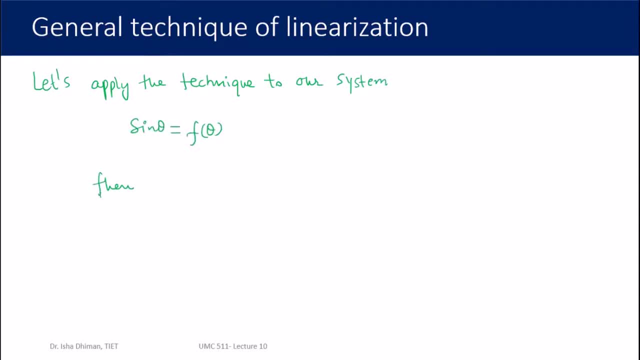 So we know that sin theta is f theta, So Taylor series expansion we are doing about the point, theta equals to 0. That's actually a Maclaurin series. So we know that x dot is fx is f dash a. That's something we just derived. 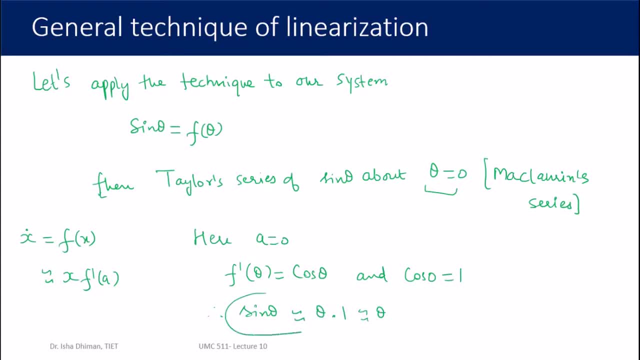 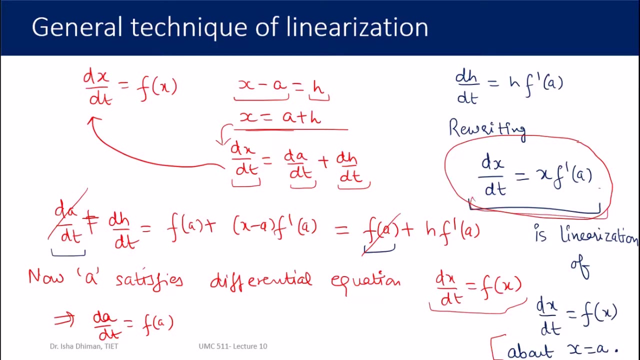 So f dash theta is cos theta and cos 0 is 1.. So sin theta is approximately equal to theta. So that's the linearization. So this is something we just derived on the previous slide. I'll just tell you this one x dot is x times f dash a.